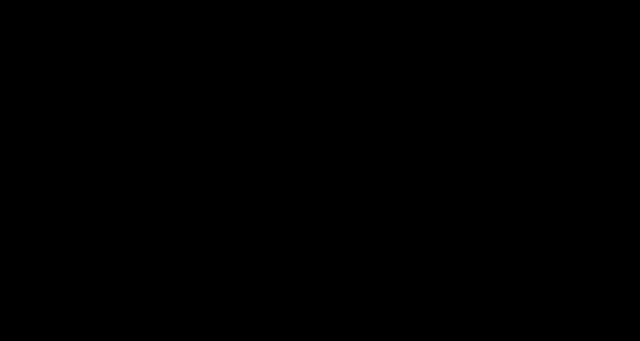 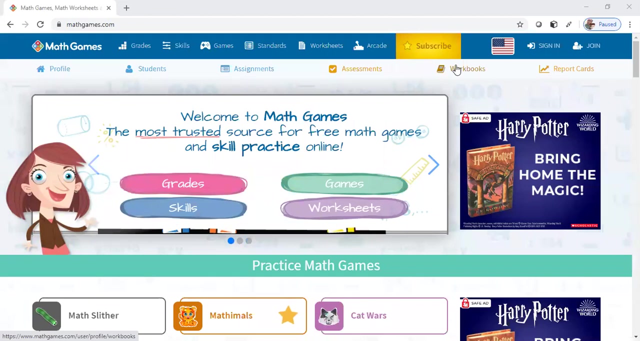 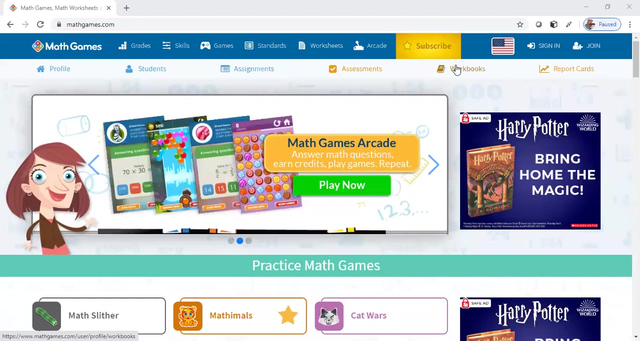 Hello guys, and welcome back to the TeacherMade channel, where everything is made by a teacher. Today we're going to talk about one of another favorite math websites that I like to use inside my classroom for my students, and this website is called mathgamescom. You can just search it up on. 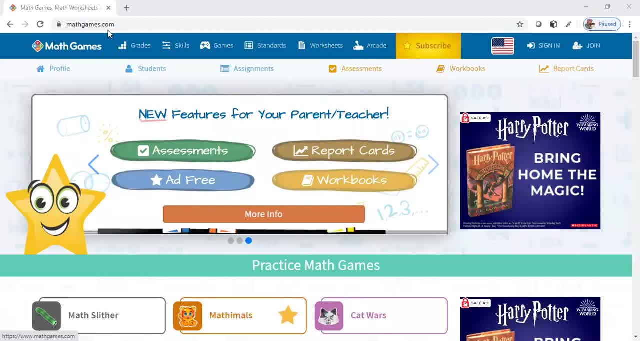 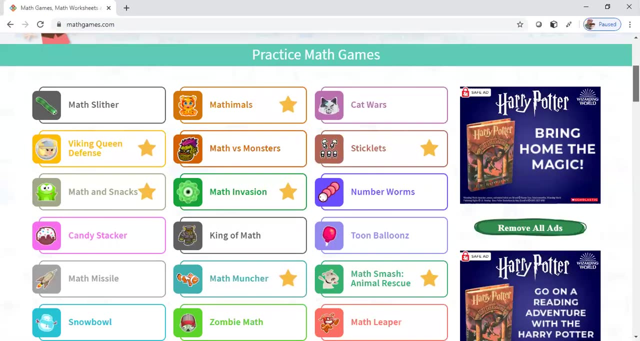 you know your student's laptop or you can project it on the board, which is what I usually do, and it's called mathgamescom. and I know what. you're probably thinking that it's all just games, and no, that is not true. They do have games on here, as you can see where it says practice math. 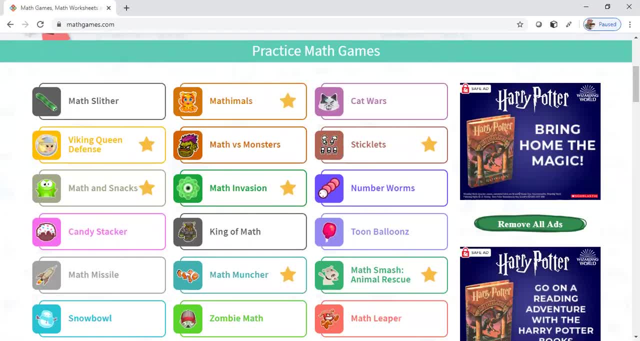 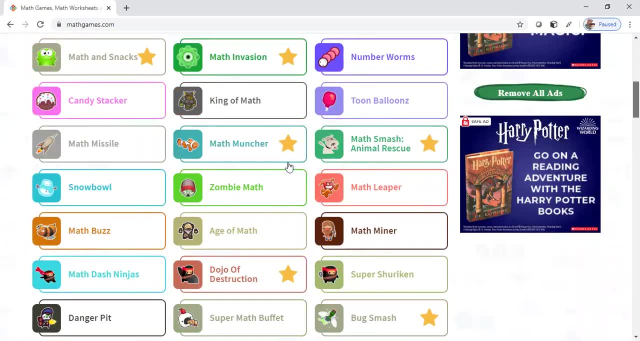 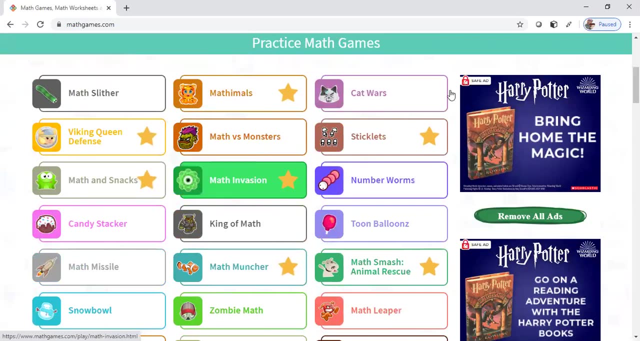 games. They have different games on here, Anything that has to do with math. these are the games listed below. One of my students favorite games to play on here is number one, And they also like the cat wars, So I'm going to take you into this website and show you why this. 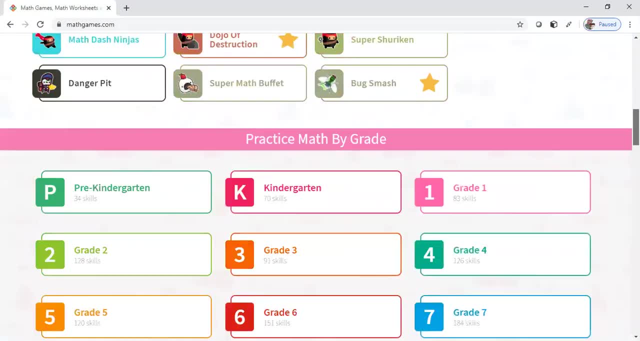 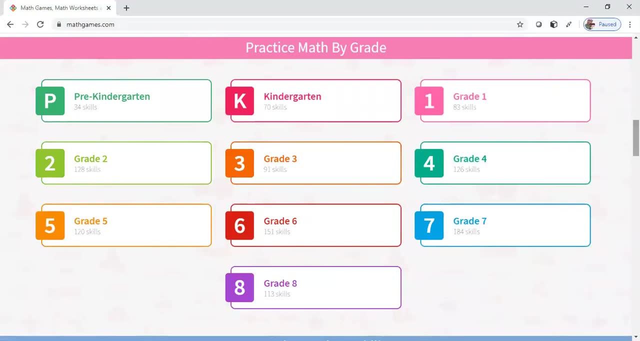 is my favorite website and something that you can probably use inside your classroom. So down here at the bottom, we have practice math by grade, and this is what I like about this website, because you can. it breaks it down by the grade level and it goes all the way from pre-k. 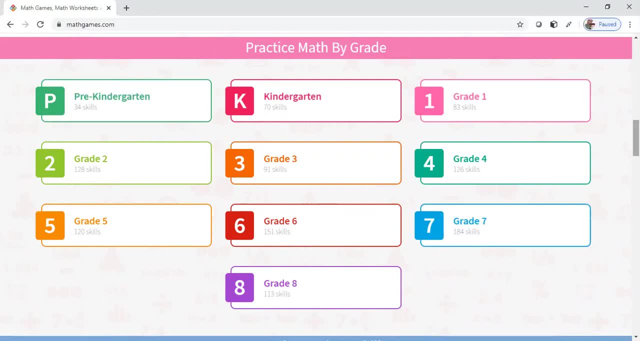 All the way up to seventh grade. So you know, if you have a student who's in kindergarten but performing on a first grade level, you can give them first grade work. So we're going to click on grade one, And what I also love about it is that it gives you the standards that goes with it. So 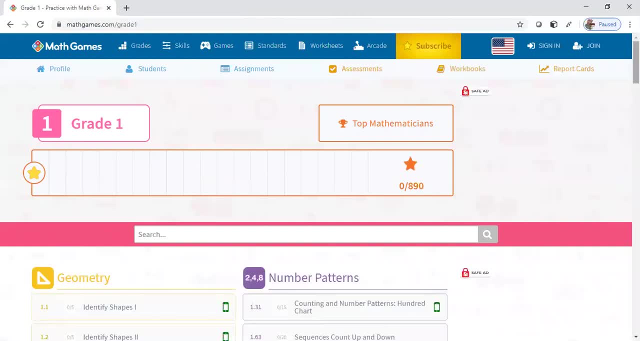 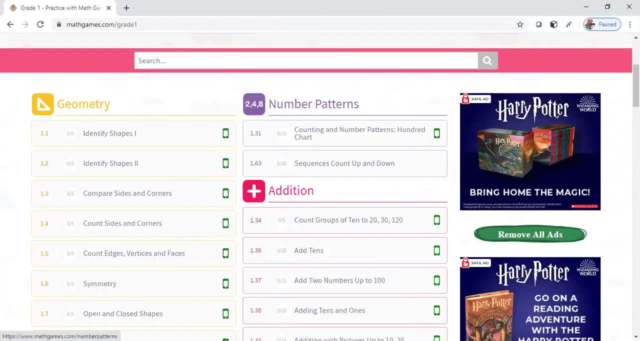 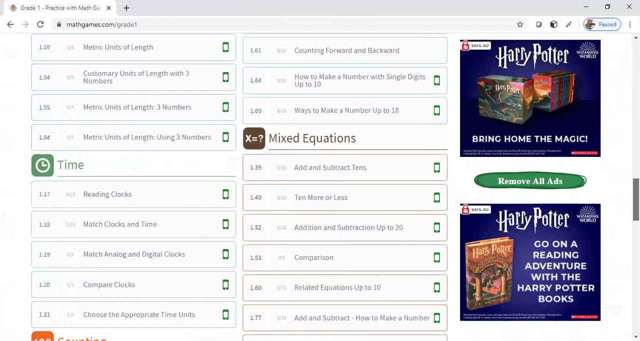 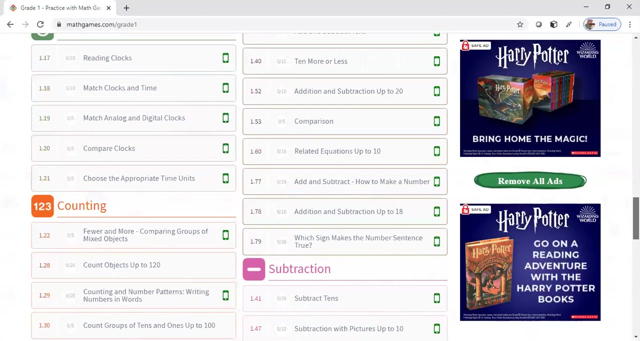 each lesson is built in with the standard, So as you can see. it's broken down into geometry, number patterns, additions, comparison fractions, number properties, measurement, mixed equations, time counting and subtraction and graphing, So as you can see the numbers next to it. these are your standards. These are your. 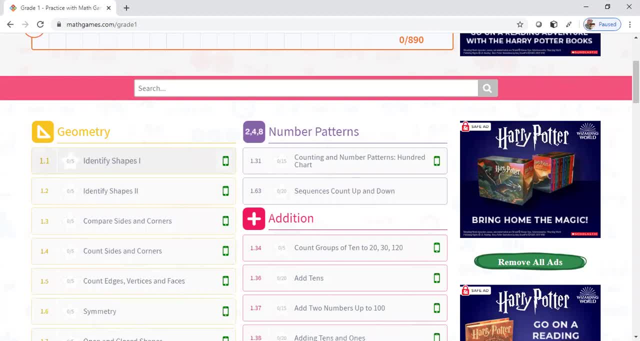 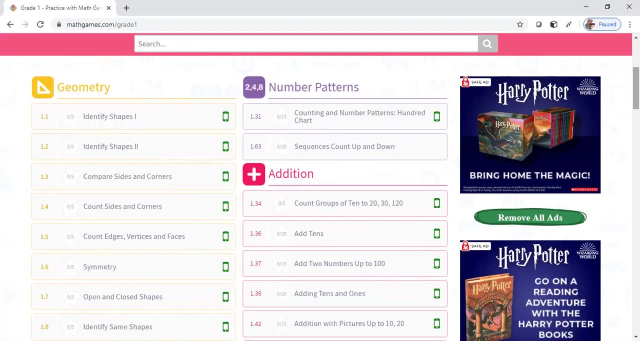 standards. So anytime you're writing a lesson plan you can put that you use- you know, independent practice for mathgamescom as a independent practice for your students and you can also put the standard next to it. So say that you want your students to work. 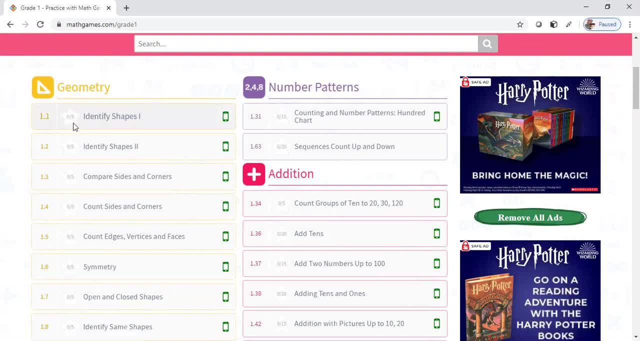 on geometry. So, and you're also going to see a star and it's going to say zero out of five or out of 15 or 20, and the student has to try and get the the star, because each student can have their own login if you create a login for them- And I'm going to show you that a bit later, but 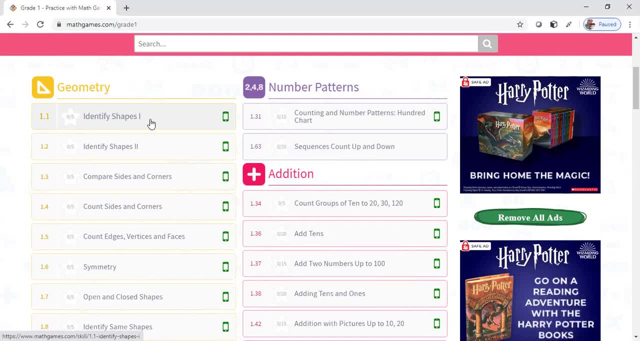 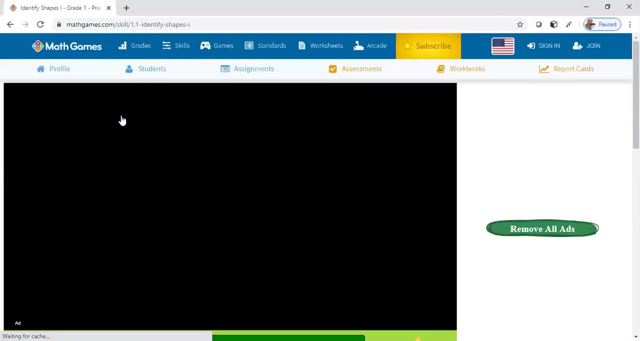 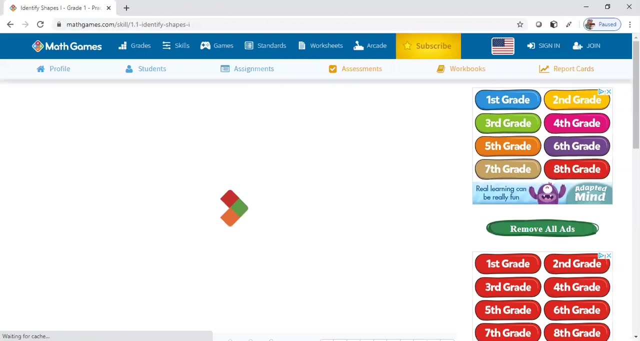 you don't have to have a login, So let me show you this example under geometry. The first one is identify shapes. So in each grade level is the same standard concept. You're just working under that grade level. So this is what it's going to look like when it comes up. So up here the student has their profile and then the 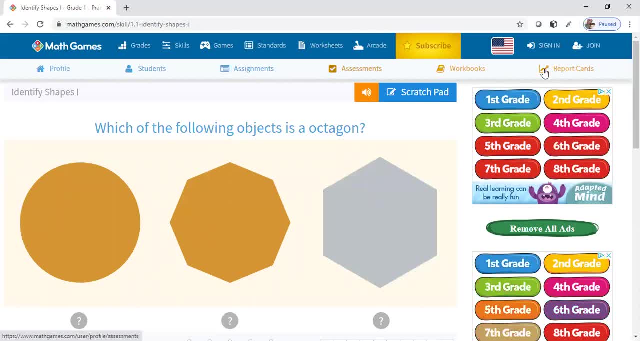 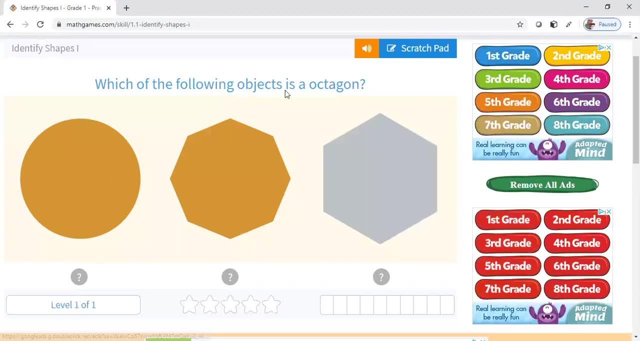 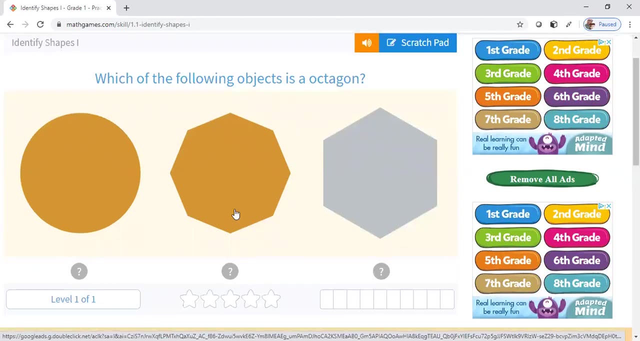 assignments you sign and then they have assessments. So you can see that they have their assessments workbooks and they get their own report card so they can track their own data. So right here it says which of the following objects is a octagon And it's going to have question marks also, As you can see. I 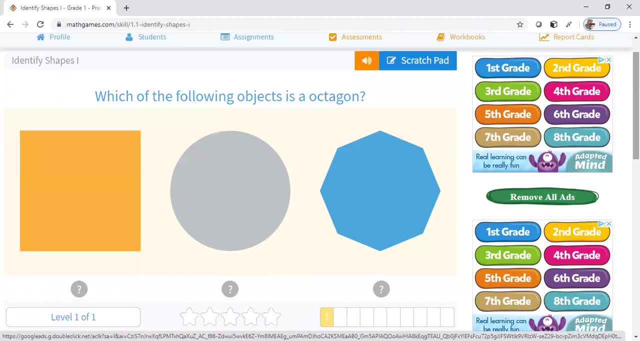 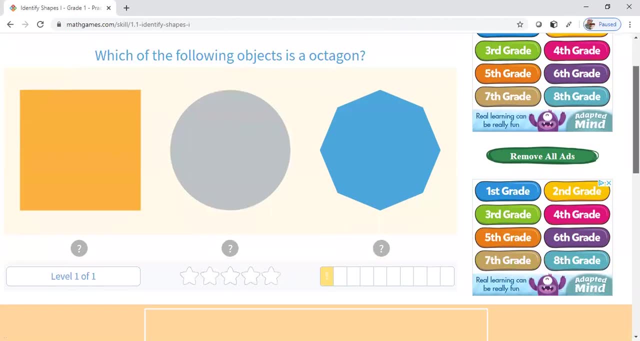 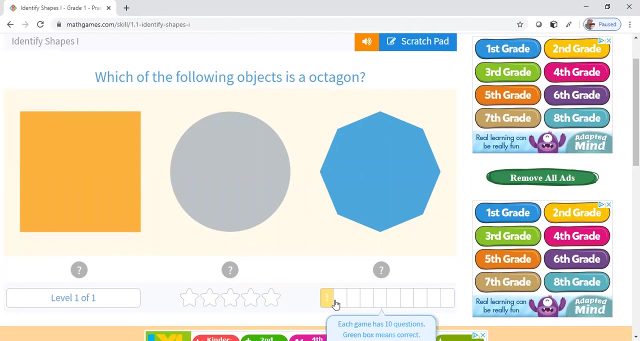 already picked the wrong one. And when they pick the wrong one it will show them an X. But when they and when they, when it, When you pick the wrong one down here, it grades itself. So if you see a yellow box, that means the student got the. 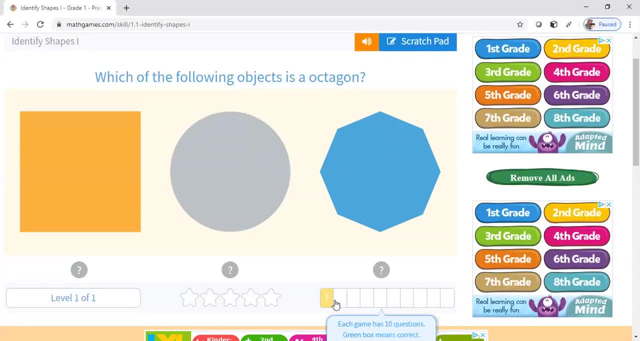 answer wrong. So that way they're checking their own progress as the same time as they're they are doing the lesson itself. So let's go back and click the correct one. We are looking for octagon, So that's what's going to happen. 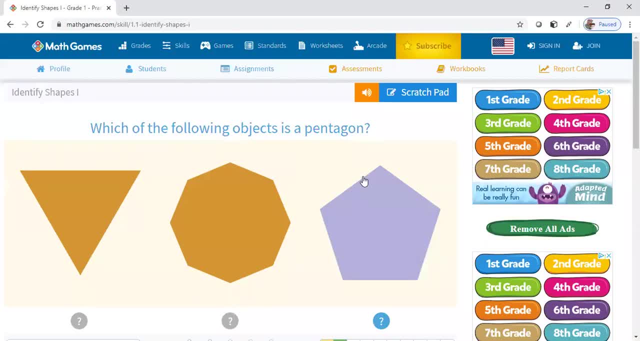 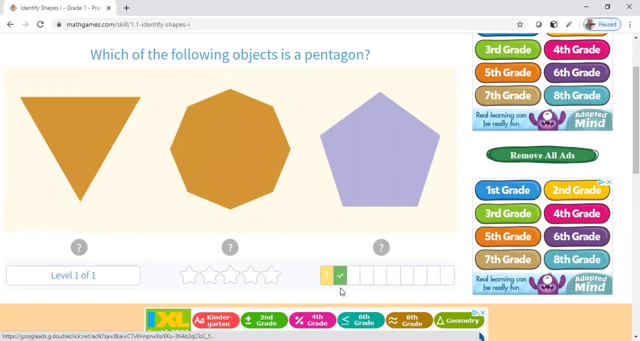 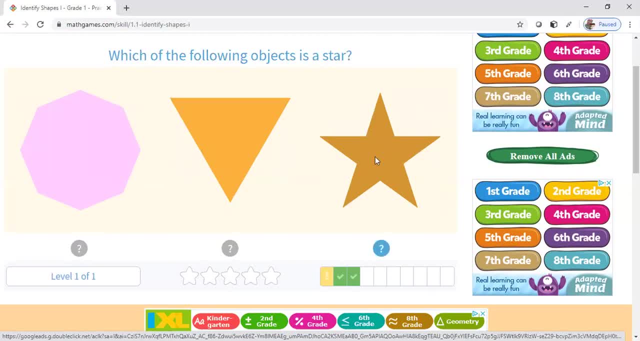 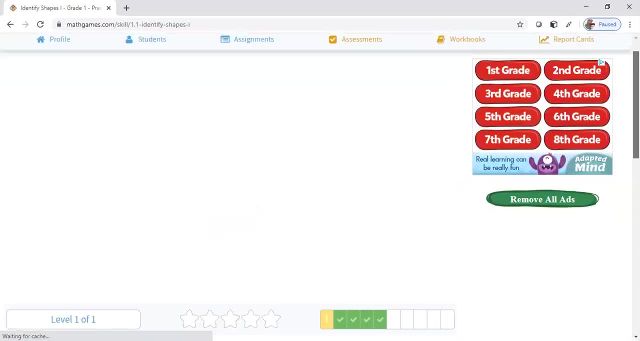 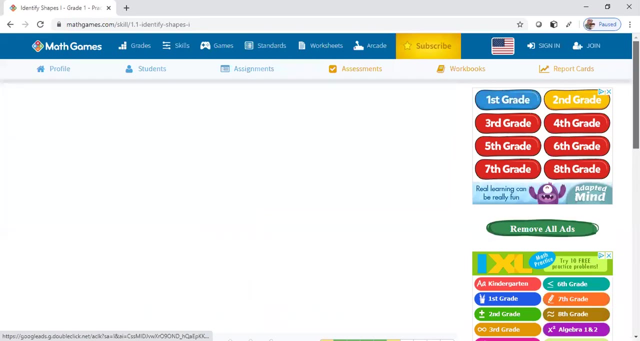 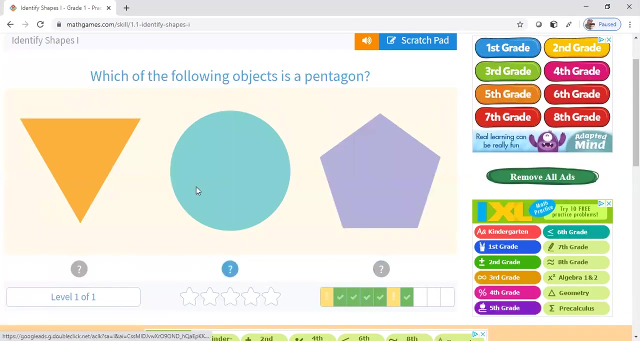 these all the way out so I can show you at the end what it's gonna look at, look like. and it's also always ten squares down at the bottom where it says where's the green and the yellow check. so we're gonna keep going. sorry about my dog. so 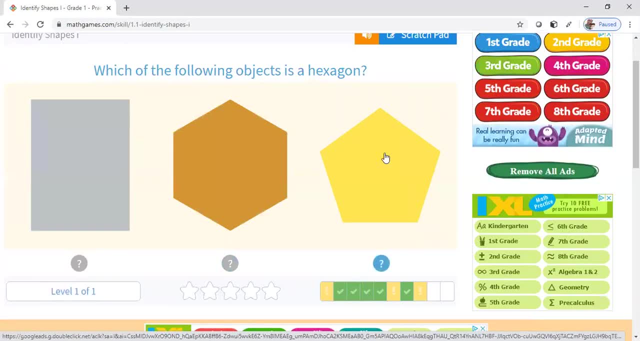 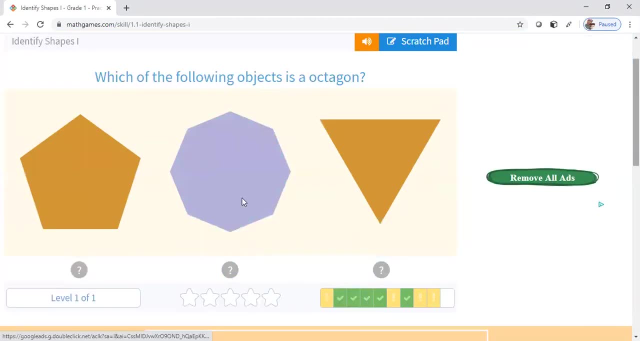 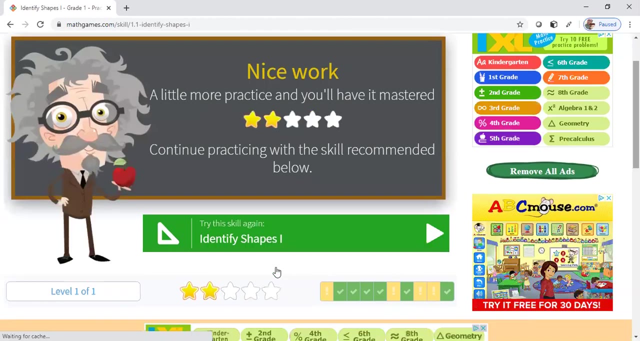 I'm gonna show you at the end what it's going to look like, and so at the end it's gonna have, like I said, the stars at the bottom. it'll have two stars out of five, because that was what the goal was, to get out of five, and then, at the 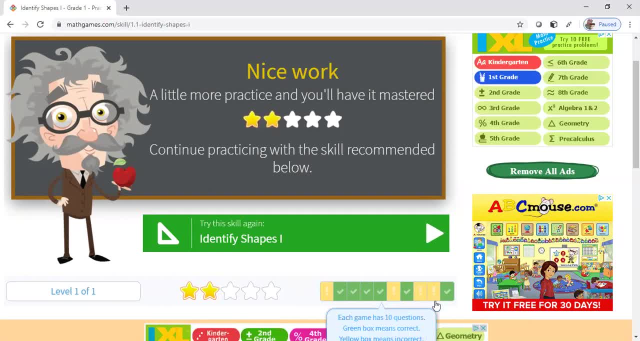 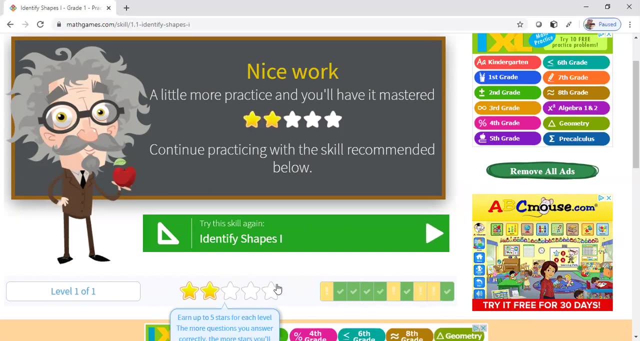 bottom it shows each student out of ten questions how many they got right and how many they got wrong. so they would do this on each lesson until they have mastered it. and if they have mastered it then all of these stars would be lit up at the bottom. so it says 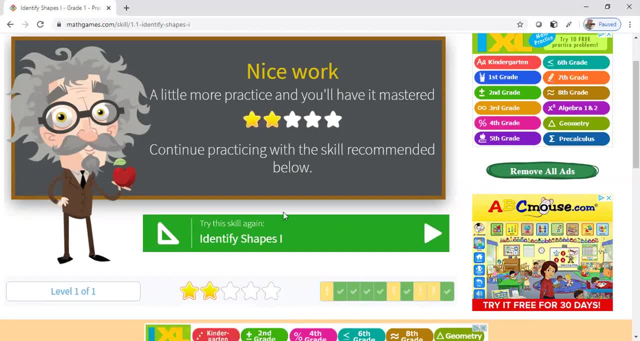 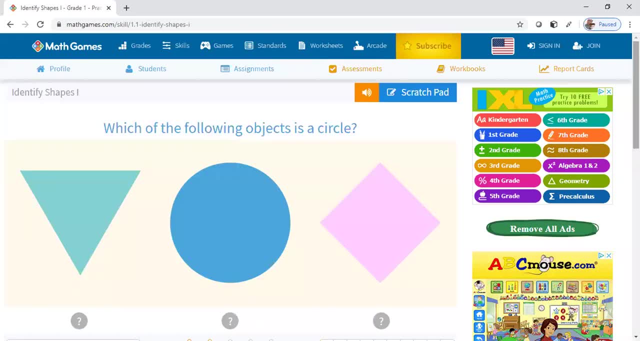 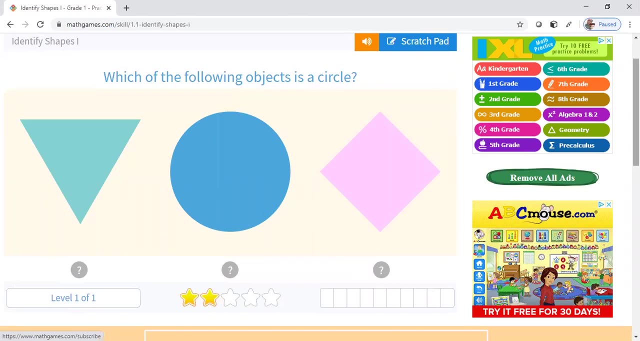 nice work. we'll do a little bit more practice. and then it moves them to the next skill. so they click on the next skill and it'll keep them on the same skill until they have mastered this skill. and they will have. like I said, all the stars are lit up at the bottom on this website. we also have it also has. 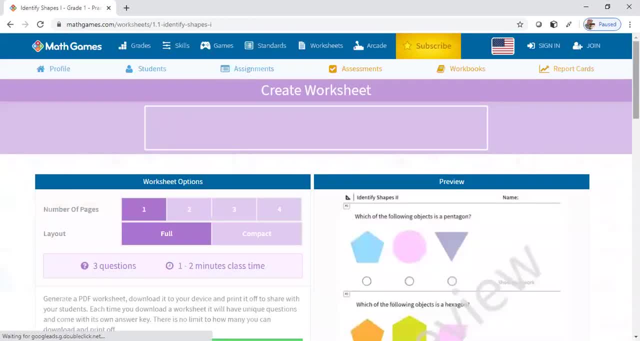 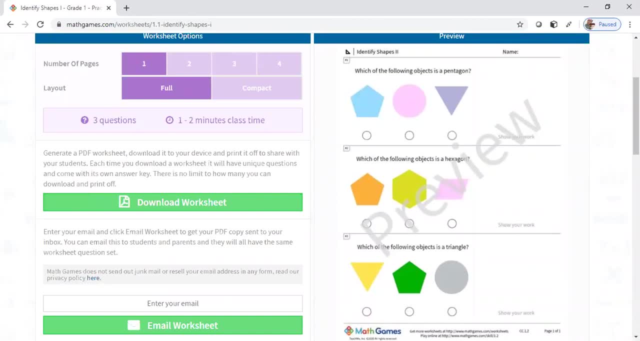 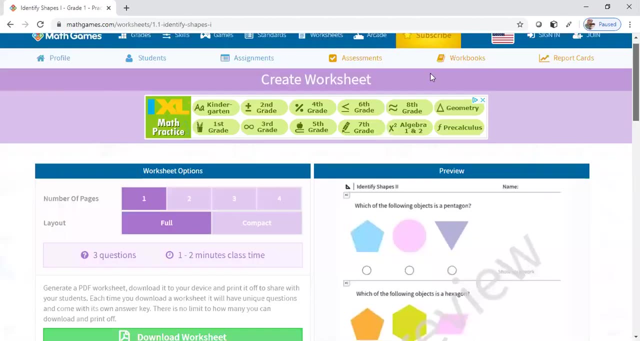 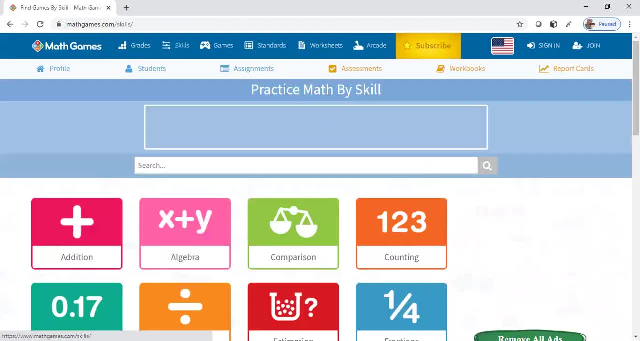 click on the next one, and then we can click on the next one, and then we can click on the skills tab, so as you can see all of the math skills tab, so as you can see all of the math skills are up there, and then we're. 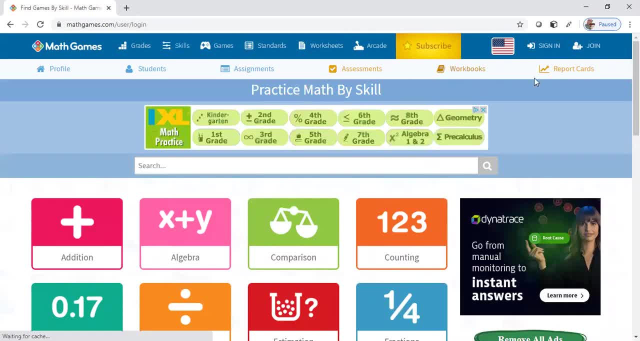 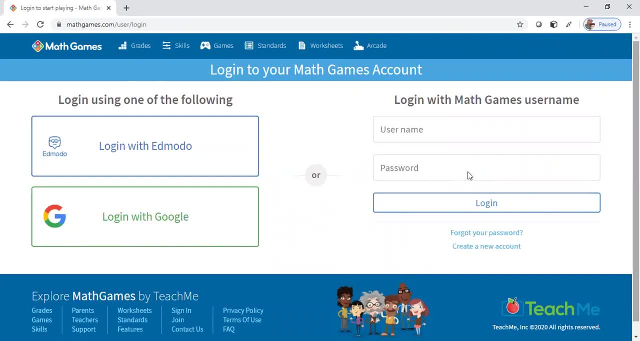 skills are up there and then we're going to go into the workbooks. okay, so for the workbooks you have to be logged in and for the login, this is where you would go, and if you click join at the top, then you can join as a.